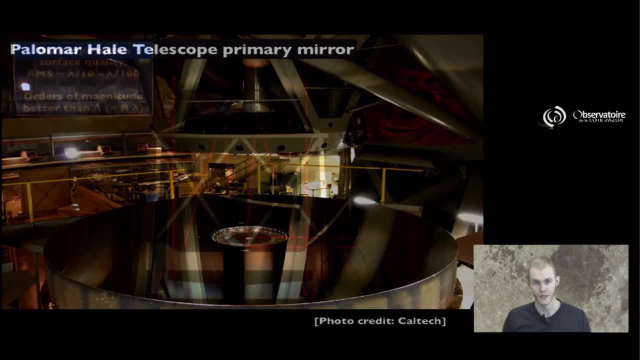 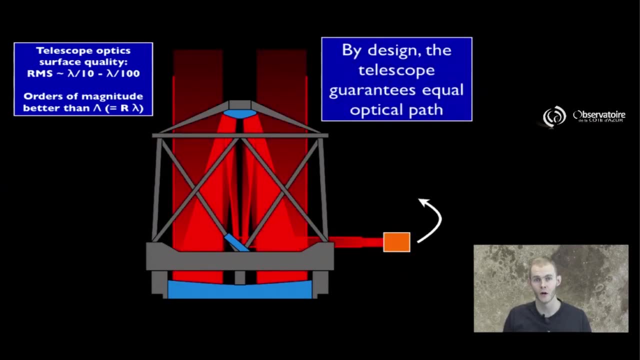 are used in imaging astronomy. In fact, if you look at most specifications for the optics that are used in everyday astronomy, you realize that the optical surface quality, the typical error, the roughness errors on the surface of the optics, is typically somewhere between lambda over 10 to lambda over 100. 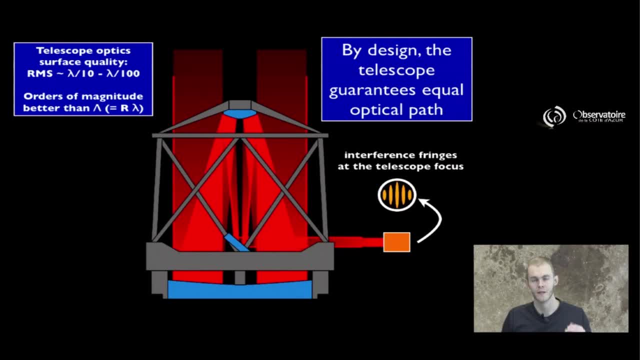 That means that the typical errors are smaller than a tenth of the wavelength, or even a hundredth of the wavelength in the most demanding cases. Now, if you compare that to the requirement we've set in order to be able to witness interferences, the constraint that was imposed by the coherence length, you realize that. 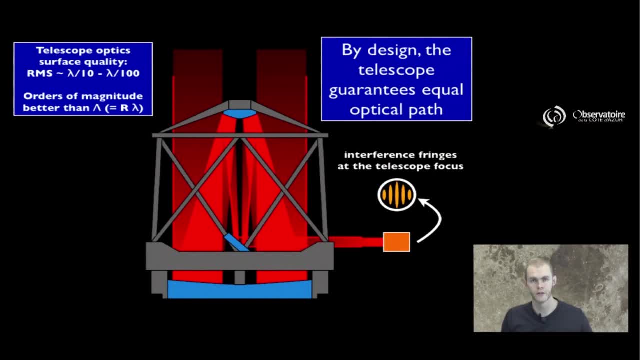 the optical quality of most telescopes is orders of magnitude better than this coherence length requirement that we've set earlier, And so it is no surprise that early day astronomers were able to produce interferences. In fact, they were able to produce interferences by simply using a telescope, an aperture mask. 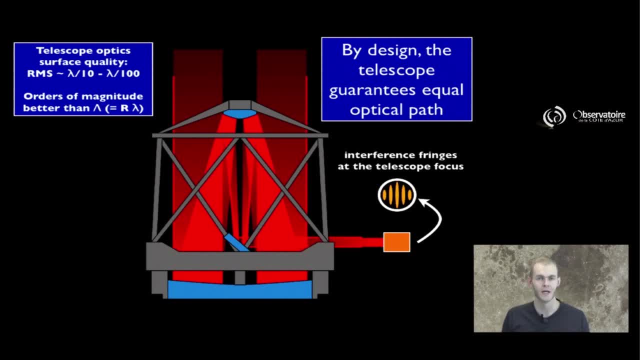 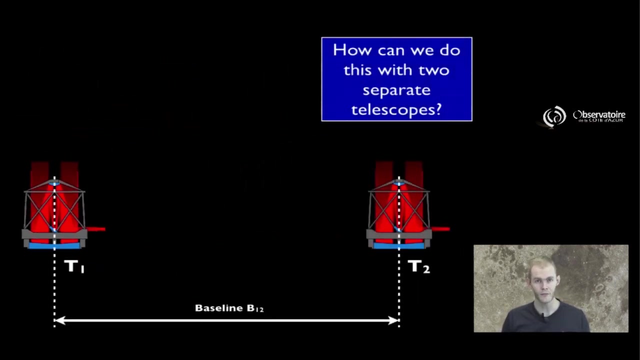 By design, a telescope is going to guarantee equal path traveled from the star itself all the way down to the detector. and if you put an aperture mask in front of your telescope, you are going to be able to observe interference fringes there. Now it becomes a little trickier when you think about trying to achieve the same thing. 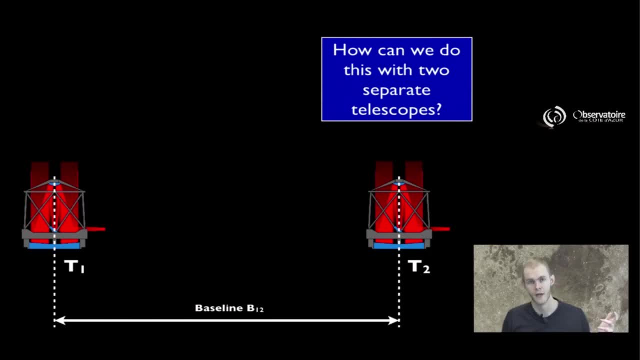 Using two separate telescopes. so here I've labeled T1 and T2, my two telescopes that are separated by a pretty large distance, that we're going to call the baseline B1-2. That can be several times or several tens or hundreds of times the size of the telescope. 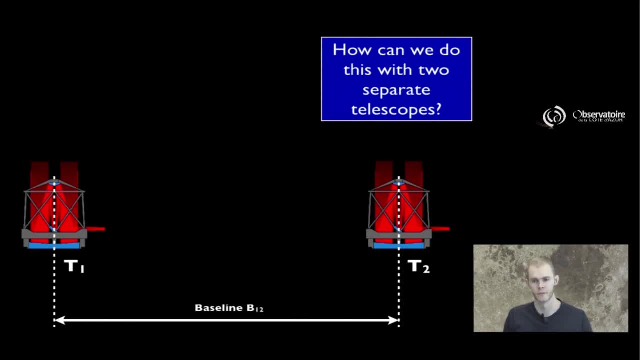 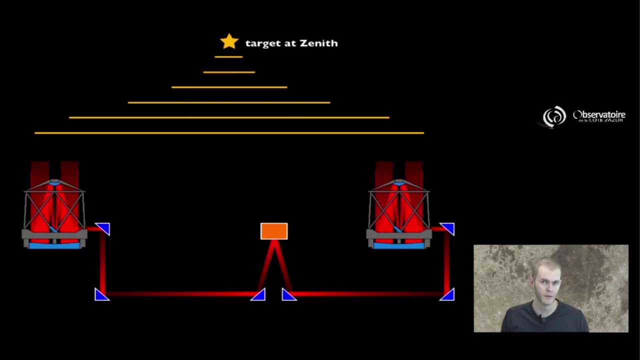 the diameter of the telescope itself. you know a few hundreds of meters. How would you proceed? The most sensible thing in order to witness, to observe interference fringes, would be to put your focal station, the instrument that is going to collect the light from the two. telescopes at the exact halfway point between the telescopes. You do that so as to ensure that the light path that is traveled by the light along the two interferometric arms is such that the light on the two arms reaches the detector at the exact same time. 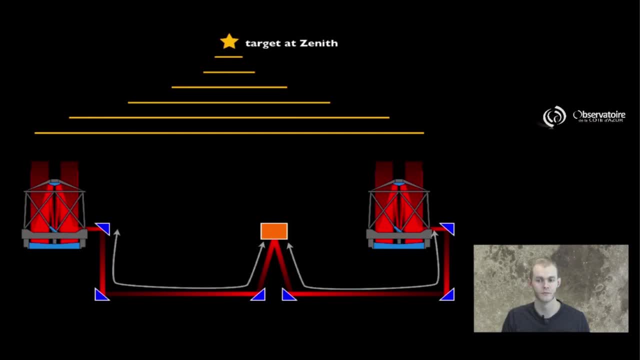 To within the coherence time, of course, And if you do so, you're going to be able to observe your interference fringes. And we're going to use a lot more optics than just the optics of the telescopes themselves in order to send the light from the telescopes to the focal station. 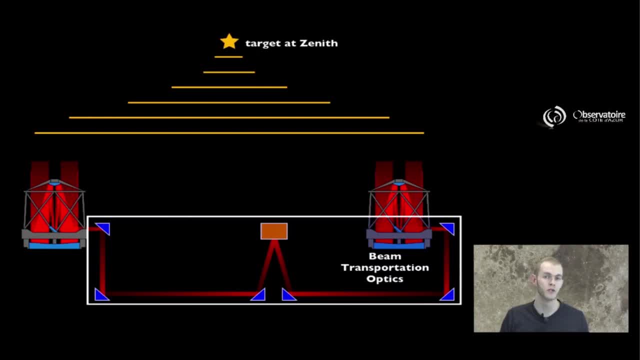 And we refer to these optics as beam transportation optics, or BTO for short. And another special place is, of course, going to be the telescope And that's going to be in the system, the focal lab itself, which we're going to cover. 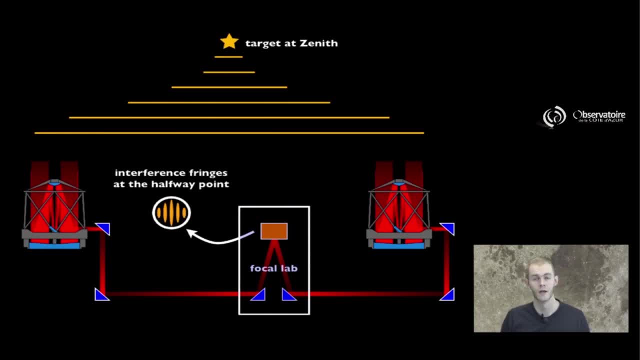 in a bit more detail in a later section. But if you do put your focal station at the exact halfway point- assuming that you're observing a target that is exactly above you at zenith- then you're going to be able to observe interference fringes at this exact halfway point. 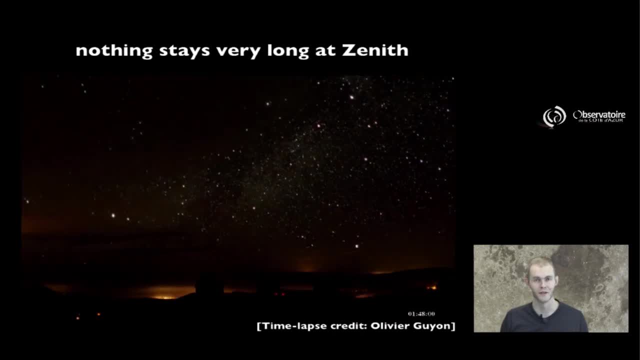 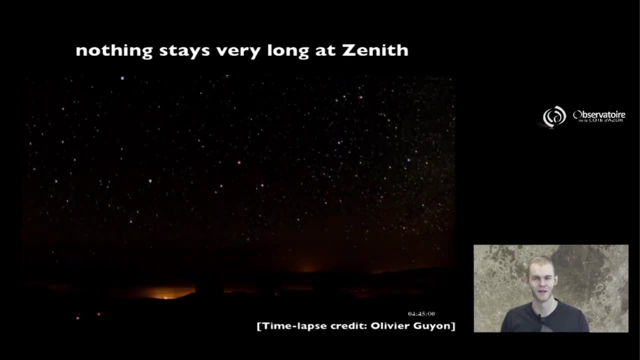 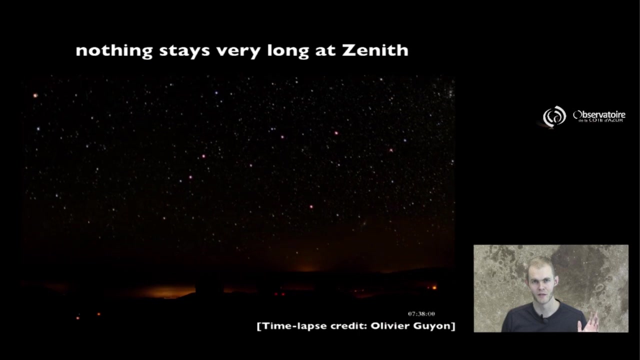 The catch is, if you've ever been out at night And looked at the sky for more than a few seconds, you know that nothing stays exactly above your head for very long, simply because the Earth is spinning on its axis As the night progresses. we simply see stars and planets and everything on the celestial. 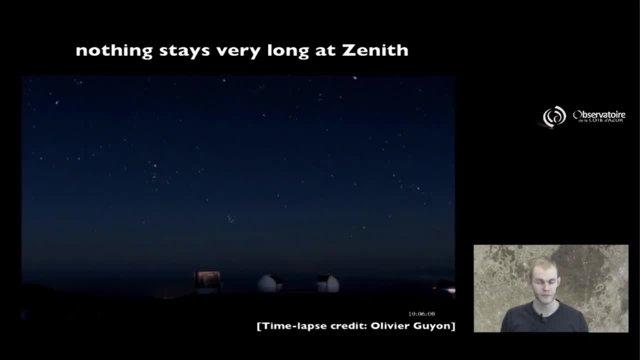 sphere drift westward, And so no object, no target is actually going to stay exactly above you, And that's what we're going to do. And that's what we're going to do, And so no object, no target is actually going to stay at zenith for more than a fraction. 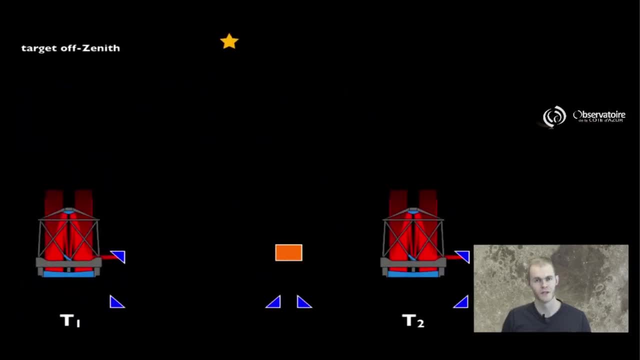 of a second really, And that is going to have some consequences on the architecture of our interferometer. If you want to observe something that is off zenith, the first thing we're going to have to do is, of course, to repoint our telescopes to make sure that we can actually couple the 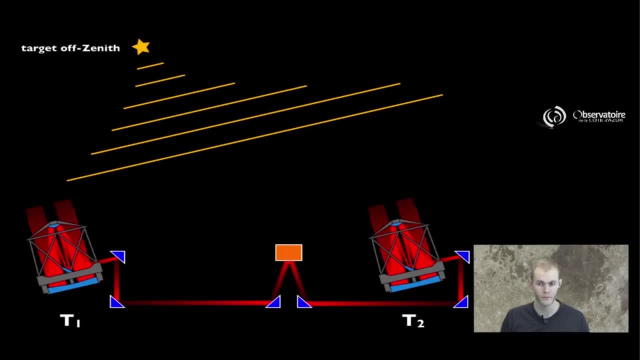 light of the star into our interferometer And although our interferometer, if we don't change anything about our architecture, we're going to not be able to see any fringes at the focus. now, why is that is? although we've ensured that the light path, 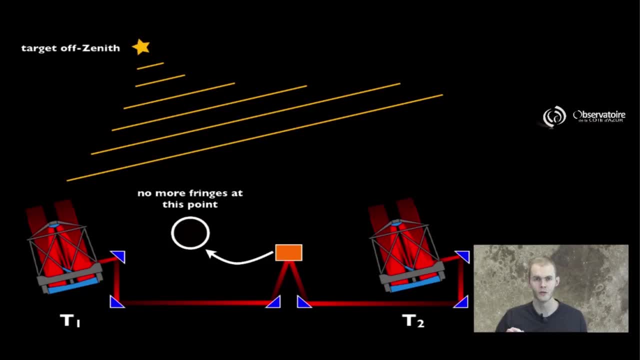 is equal along our interferometric arms. by changing the pointing, we introduce an additional optical path difference on one of the telescopes. if you look at the yellow lines that are printed on the drawing here, you're going to see that the light of the target reaches telescope t1. 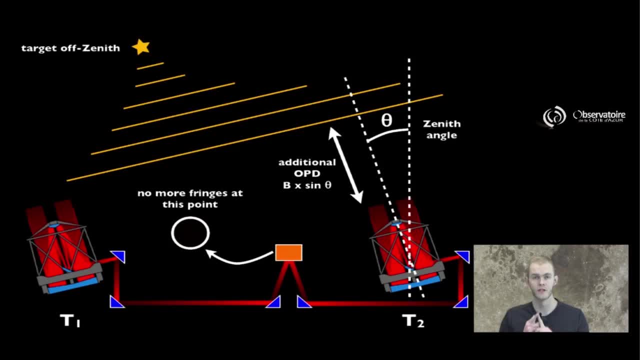 before it reaches telescope t2, and the fact that there is a very long distance between our two telescopes is such that the optical path difference this introduces can be very large, up to tens or even close to 100 meters in some cases, if you try to point very far away from zenith. 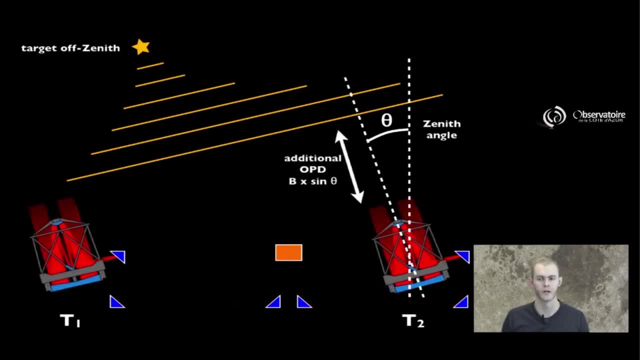 how do you address this? you're going to have to change your architecture and introduce, on one of the arms of your interferometer, an extension that it's going to delay the light by some amount that exactly matches the optical path difference that is introduced by the pointing, and in doing so you're going to make sure that the light again reaches your focal point. 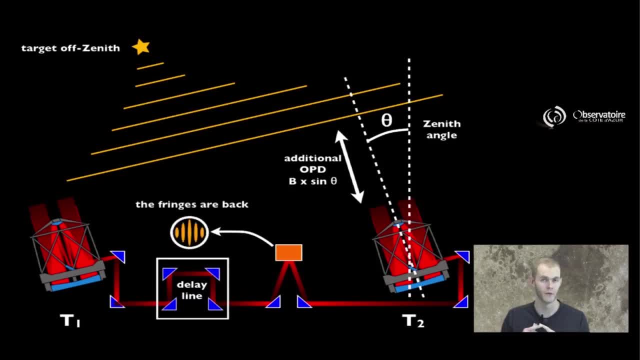 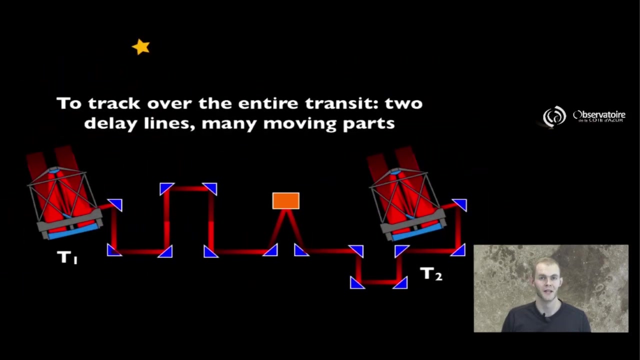 at the exact same time on for the two interferometric arms and in In this case, you're going to recover your fringes. We call this additional light extension a delay line, and this, of course, needs to be adjusted as the pointing changes as the objects move across transit. 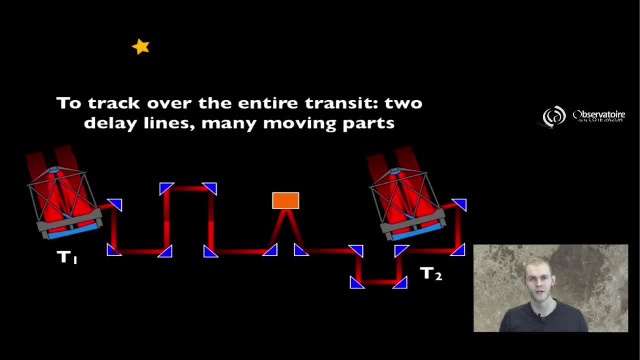 And, of course, if you want to track over the entire transit before and after the target you're interested in observing crosses the meridian, then you're going to have not just one but two delay lines and many moving parts in order to make sure that, as the star, 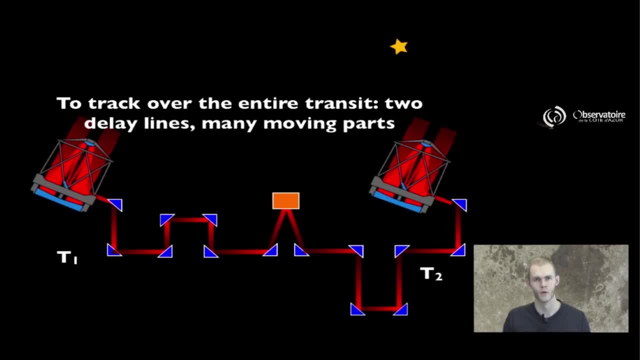 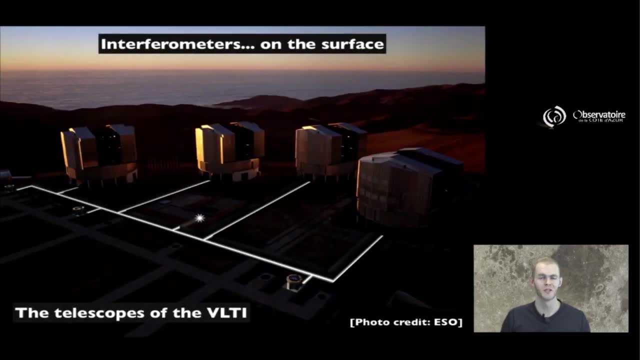 crosses the sky. you are maintaining equal path on the two interferometric arms. If you look at pictures of interferometers, usually you only think of the telescopes that make up the interferometer. But on the surface now, once the light is collected by these telescopes, what is hidden? 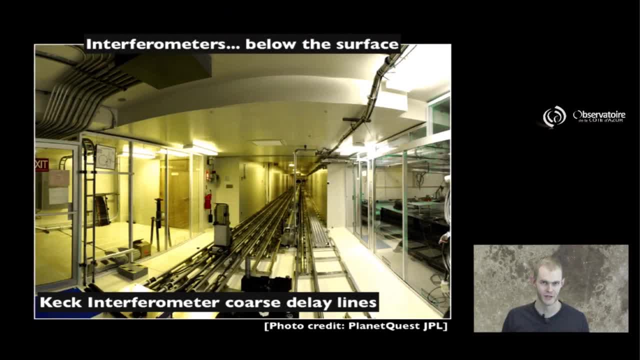 is the long tunnels that are used to maintain this equal path requirement here, And here's an example of the Keck interferometer delay line, which is a very long tunnel over which some trolleys are running pretty fast As the pointing of the telescopes changes. 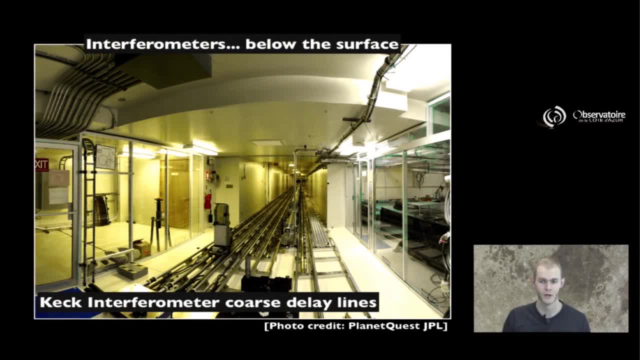 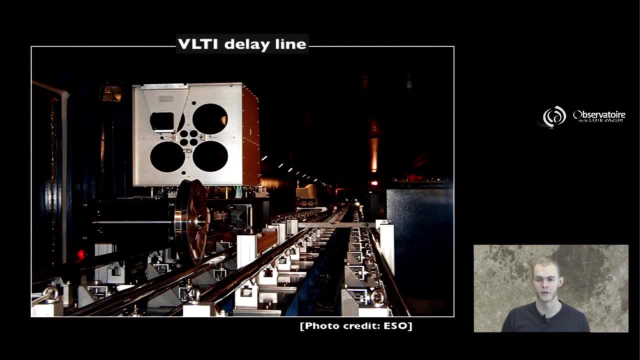 When they are operating in interferometric mode and you have the same sort of installation, of course, at the VLT-I, And here you have a picture of the actual trolley going over the long track. that ensures that we're going to maintain optical path difference. 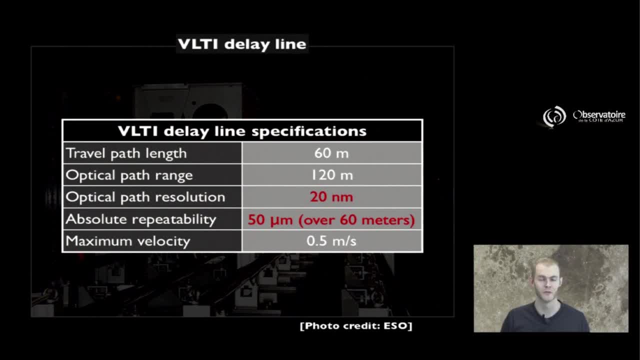 And if you look at the specifications for these delay lines, you realize that it's pretty amazing technology there. For the VLT-I example, the delay line specifications are a total travel path of about 60 meters for the trolley itself, which, if you account for the fact that the light goes back and 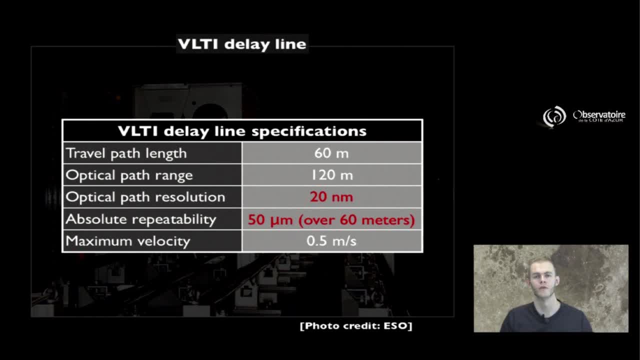 forth makes for an optical path range that goes from 0 to 120 meters tops. You have to do this with a very good resolution And, Yeah, Using the fine correction systems that they have on the trolley, you can actually maintain. 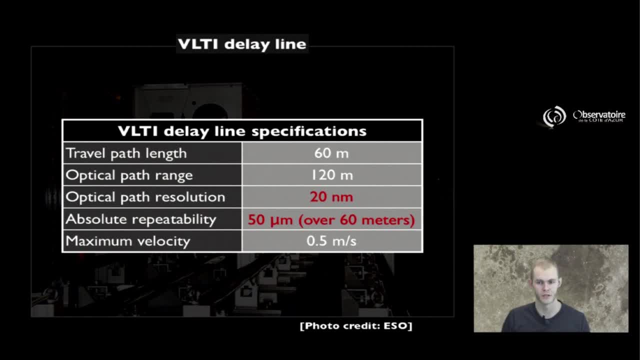 an optical path resolution of about 20 nanometers. in some cases, You have very good repeatability of the system, and if you do the applications, you'll realize that this trolley needs to move pretty fast, and so this system is designed to accommodate. 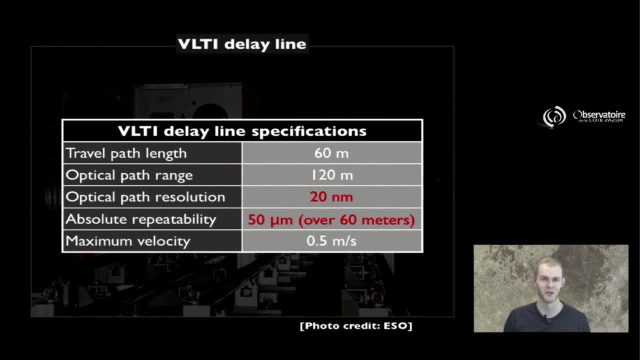 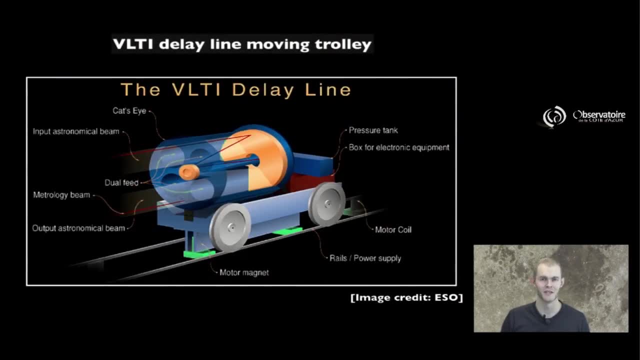 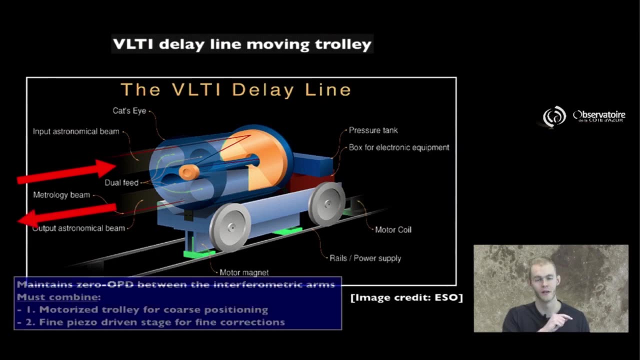 displacements. that goes as fast as 50 centimeters per second, which is pretty impressive. The trolley itself is very interesting. It is a system designed like a telescope, with light coming in and light getting out of it, making sure that the trolley itself is going to move along its track, and that's.